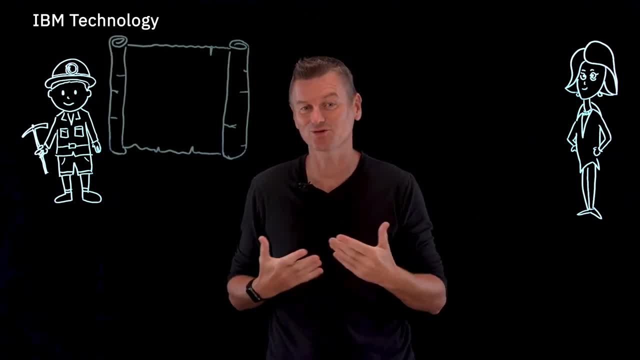 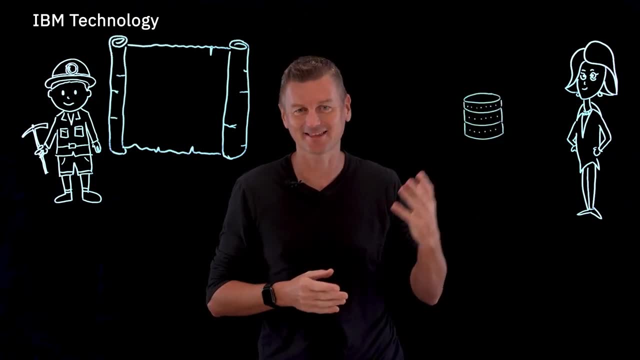 Nate, our treasure hunter, starts out by identifying a potential treasure trove location. In the same way, Sophie, the data scientist, starts by identifying a data set that looks promising. Nate, he then scopes out the area. Thecan you work there? 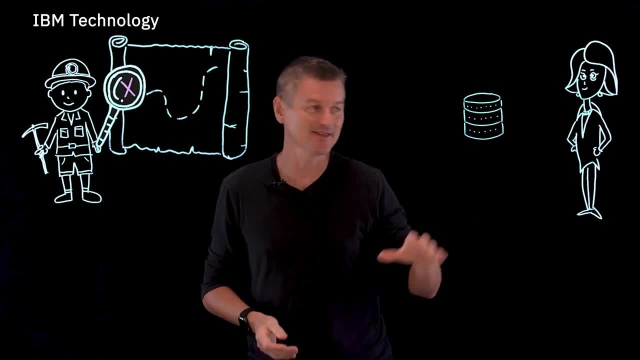 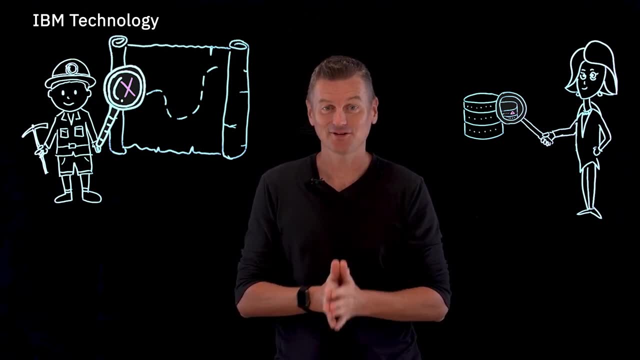 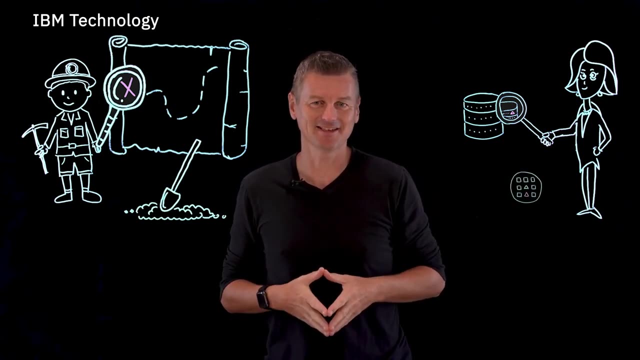 Looking for clues that there is indeed treasure to be found. And in the same way, Sophie looks at the dataset, looking for patterns or anomalies that could be exploited. Our treasure hunter then starts digging, looking for the treasure. The data scientist starts manipulating the data, looking for hidden patterns. 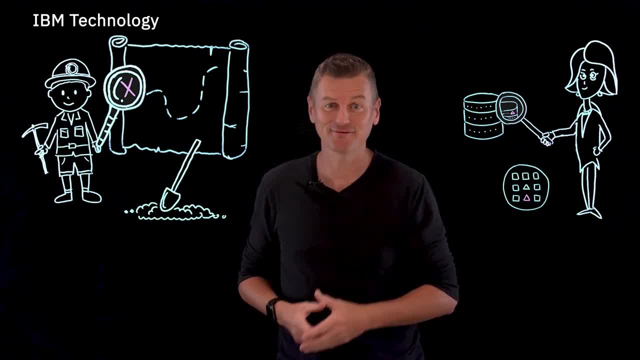 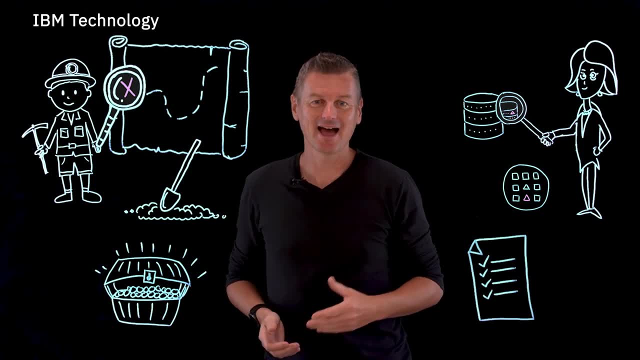 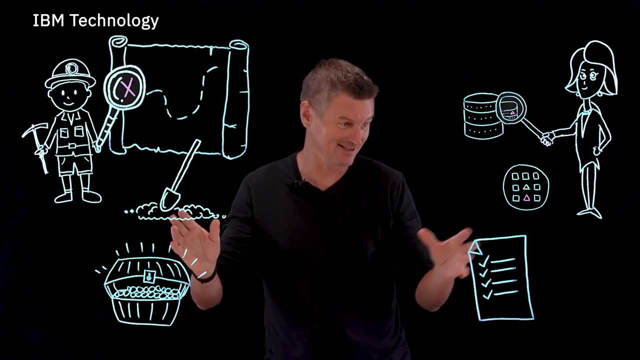 And finally, on a good day, Nate finds the treasure and brings it back to be enjoyed. And Sophie, Well, Sophie finds the insights from the dataset and brings them back to the business to be used. So, when it comes to finding what they're looking for- treasure and insights- 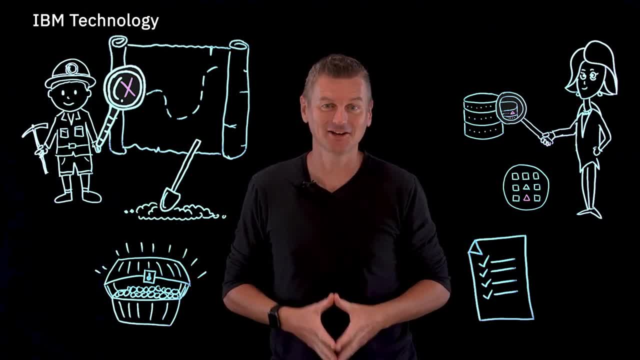 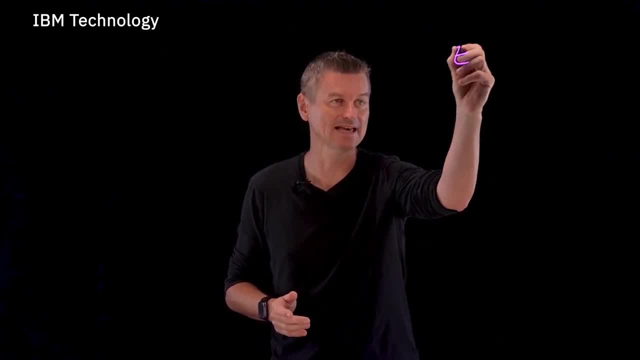 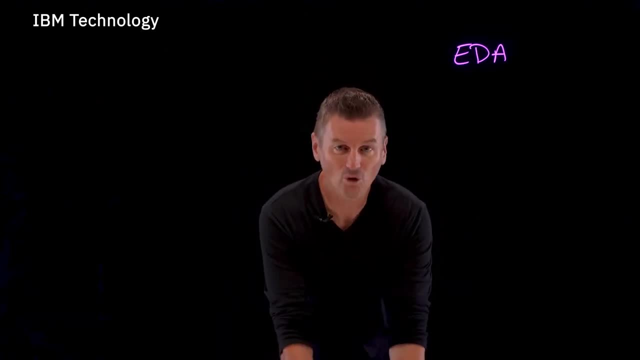 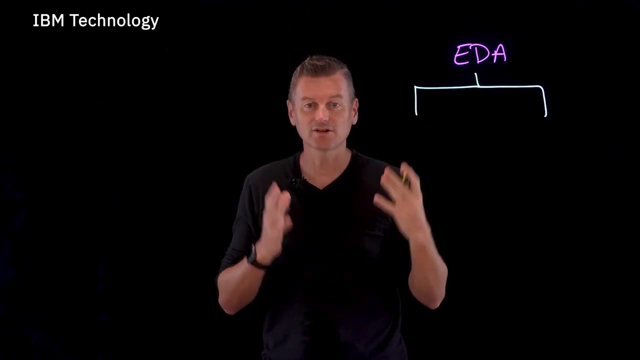 you could say that Nate and Sophie. well, they have a lot in common. So the main purpose of exploratory data analysis, or E D A, is to analyze and summarize data sets. Now there are four primary types of EDA, which we can classify into two subgroups. 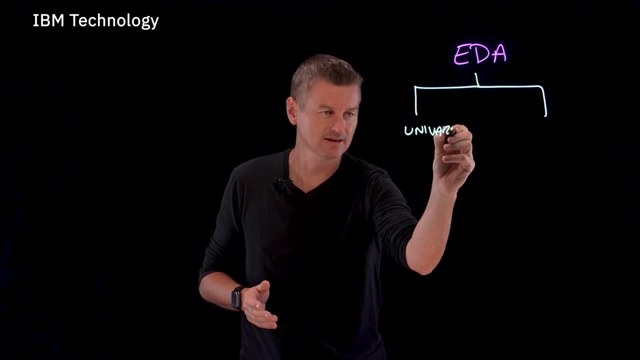 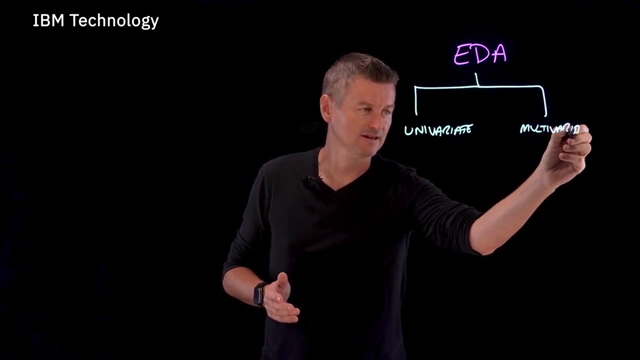 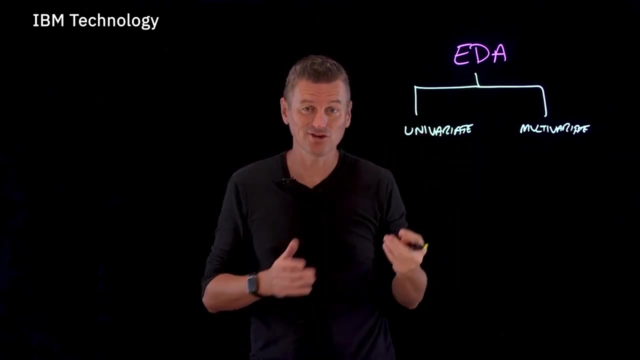 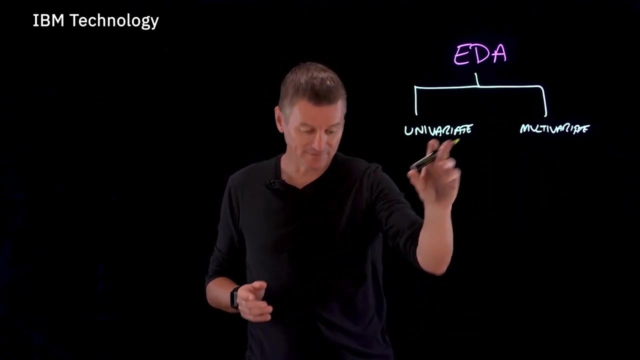 So there's univariate as the first subgroup and then there's multivariate as the second subgroup. Univariate data is data that can be described just using one variable, while multivariate can be described using multiple variables. Now, within univariate, 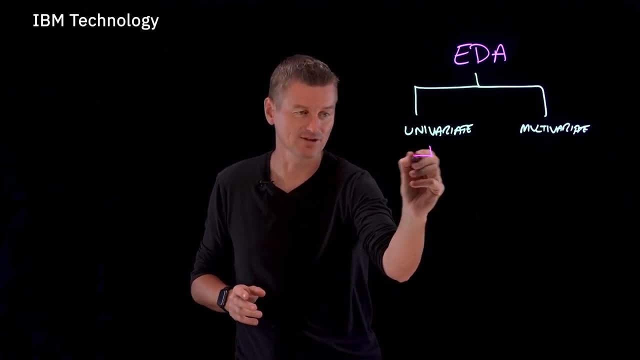 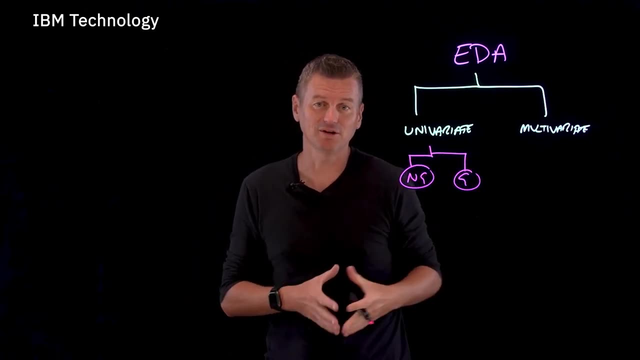 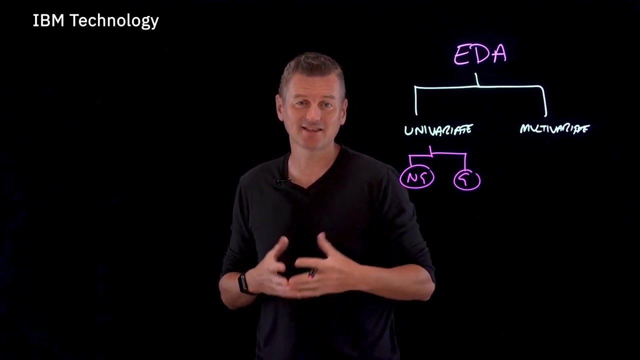 there are are actually two other classifications: There's non-graphical and graphical. The main purpose of univariate analysis is to describe the data and find patterns that exist within it And, since it's a single variable, it doesn't deal with causes or 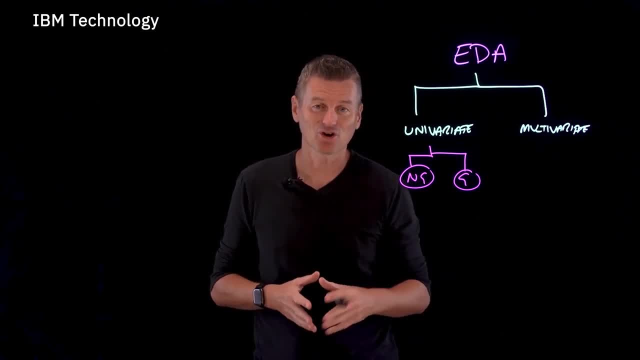 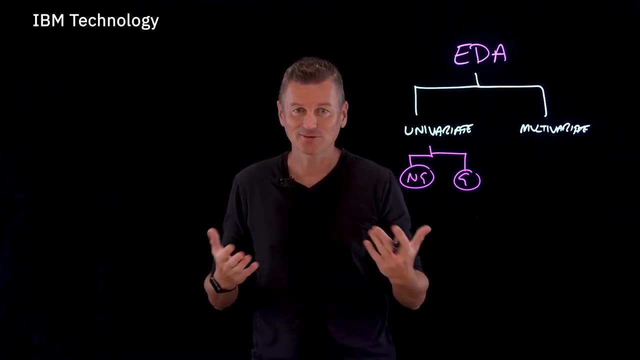 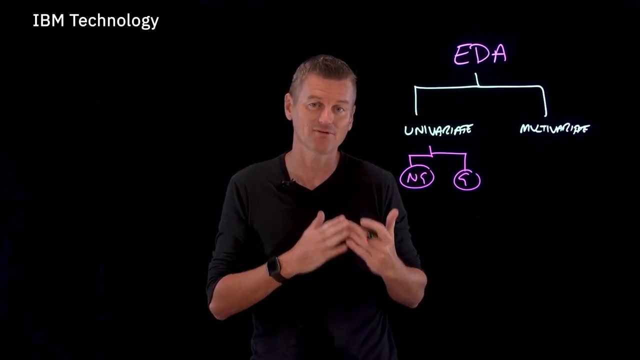 relationships. Now, common types of univariate graphics include stem and leaf plots, which show all the data values and the shape of the distribution, And there's also histograms. That's a bar plot in which each bar represents the frequency or proportion of cases for a